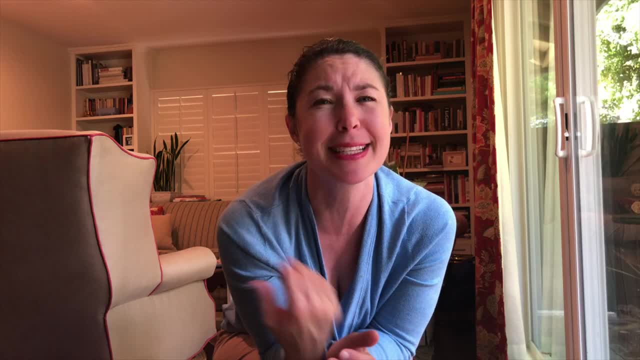 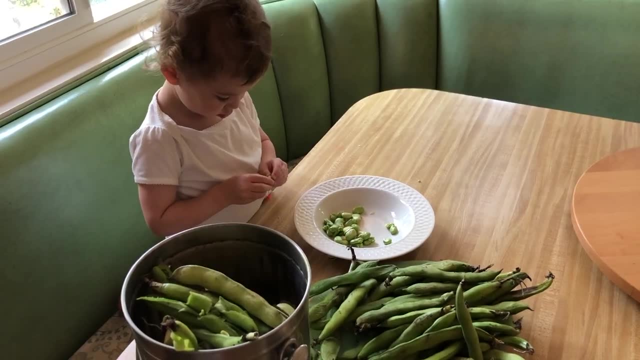 jackets, And then she told me that my job was to cook them. I feel like it's kind of an old fashioned memory that some of us have snapping string beans, shelling peas, what have you? But in addition to that wonderful, fine motor practice that it gave my daughter, it was also bonding time. 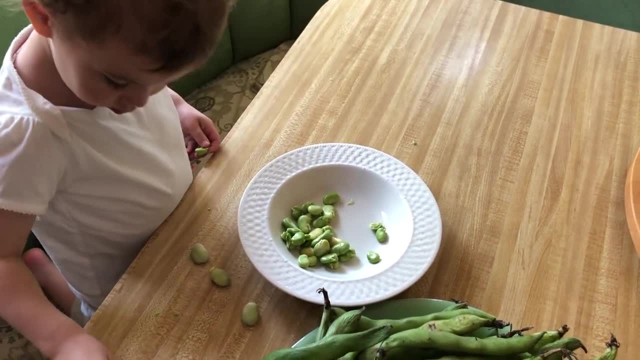 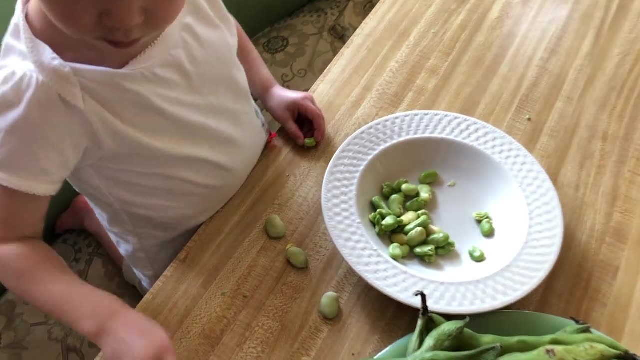 for us And it was also, you know, it was a lot of fun for me to be able to do that. So I feel like I would say like a plant learning time for her, because the anatomy of the fava bean itself is really interesting. There's a lot of parts to it and they're very oversized and big, So you're able. 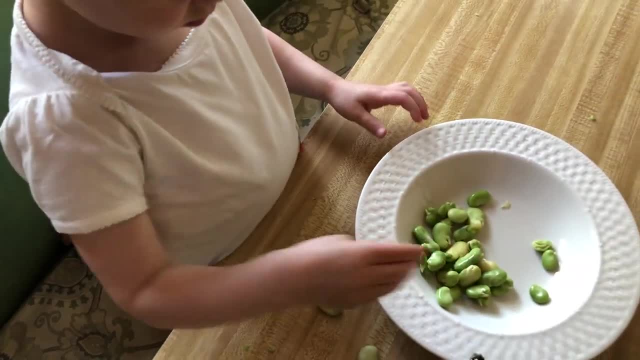 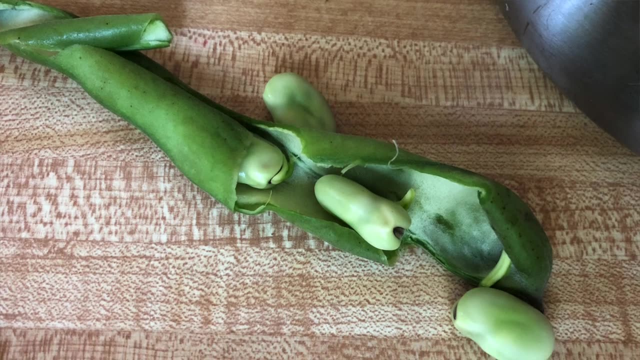 to see the pod, the way that those seeds attach to the pod, and then the various parts and jackets that come off, and even where the seed will ultimately sprout from. So they were really interesting objects in themselves, even if they are not a food that your family consumes a lot of. 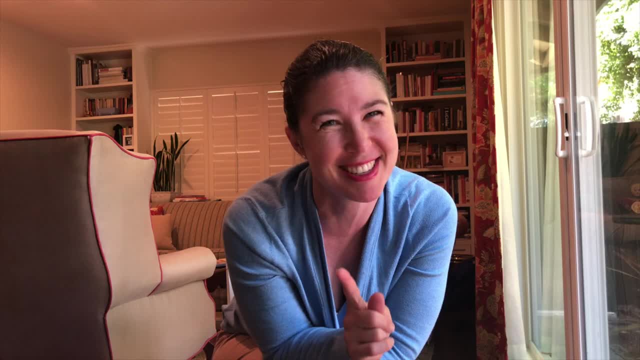 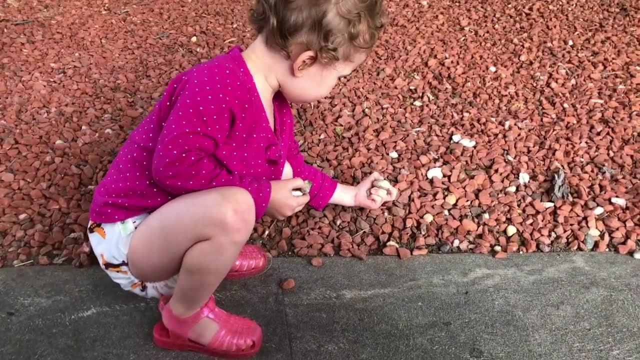 The second activity that does not require your own house- because this wasn't at our house- is rock sorting. I'm sure that many of you have areas that you go by where there's gravel And in some cases, like in our neighborhood, 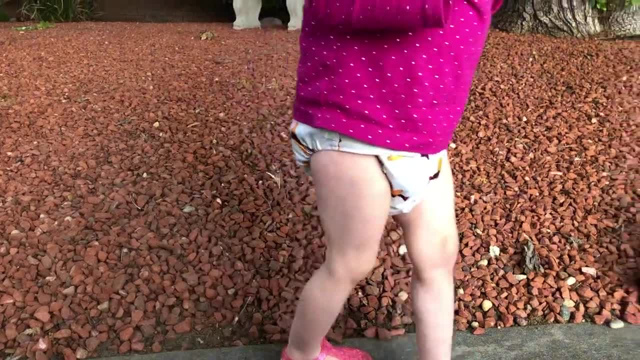 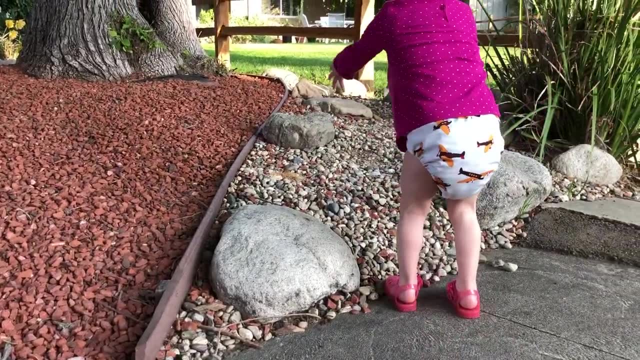 we have neighbors who have two different kinds of gravel in different flower beds or areas along the sidewalk. This week, while taking a walk, my daughter took it upon herself to sort the rocks, which means that when someone walks by and kicks up a rock, sometimes the colors intermix. 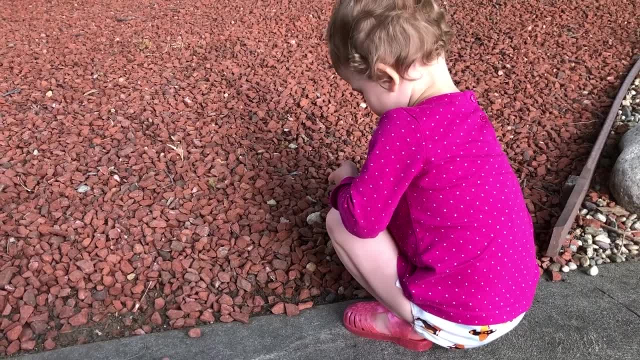 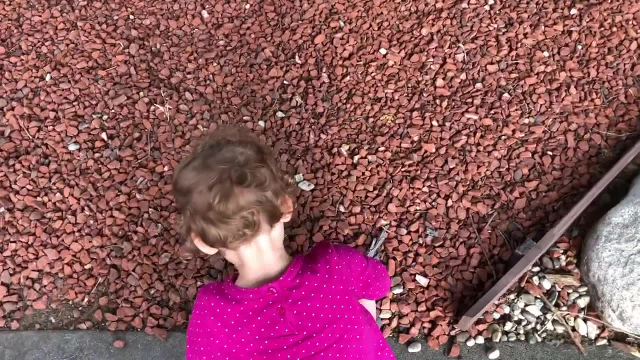 And so, just like a shape sorter or a color sorting activity that you might do with a nursery school aged child, this was a cleaning up job where she took it upon herself to separate the white rocks from the crushed brick and she could easily tell the colors apart. and 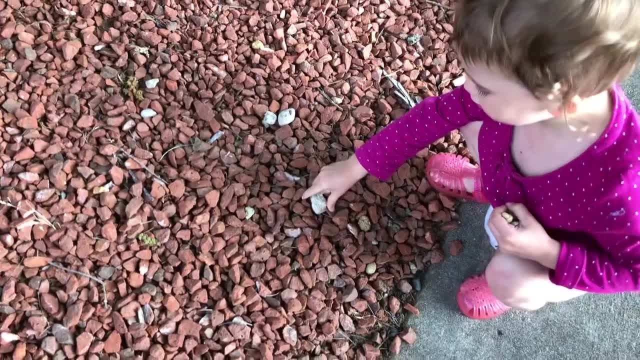 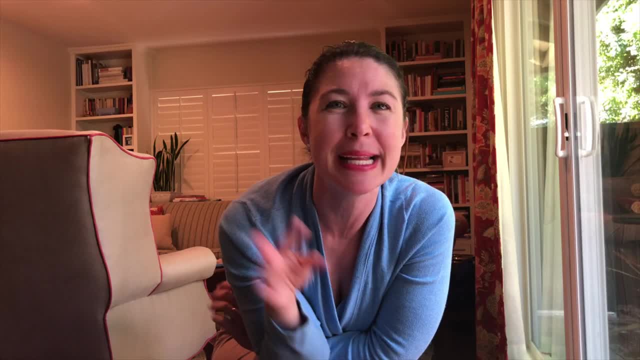 put everything back in its place And she easily spent 15 minutes putting things back together in our neighbor's yard where the rocks had gotten intermingled and mixed up. Those are two nature outdoor activities: one with organic seed pods and the other one with 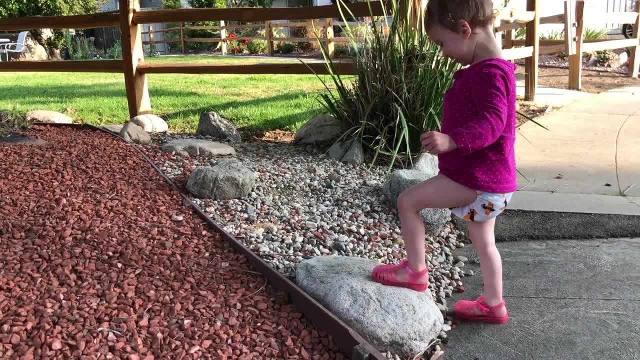 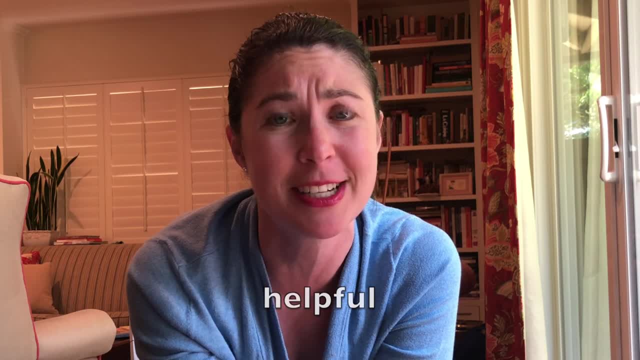 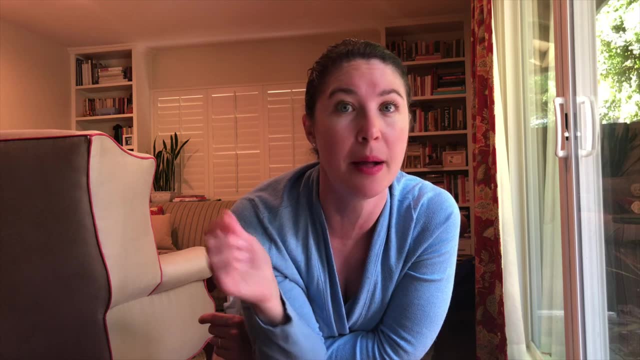 rocks, which are kind of an interesting material To look at and learn from. both of them involve fine motor skills and decision-making. Both of them were helpful things that my daughter did And both of them kind of tap into the desire to manipulate small objects or loose parts And I can link a book to that down below If you're.